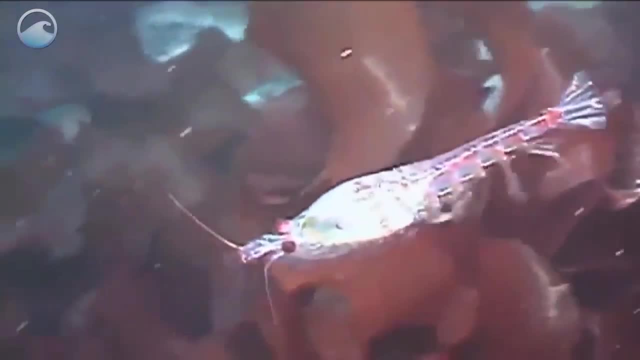 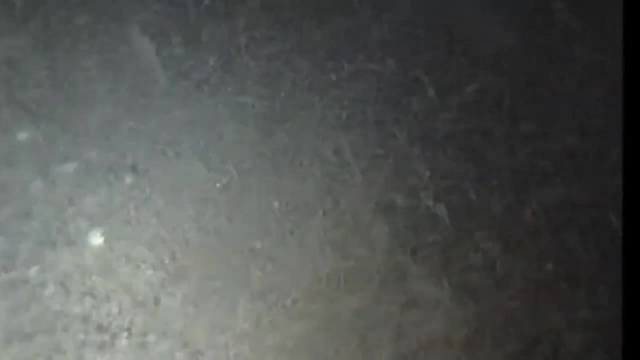 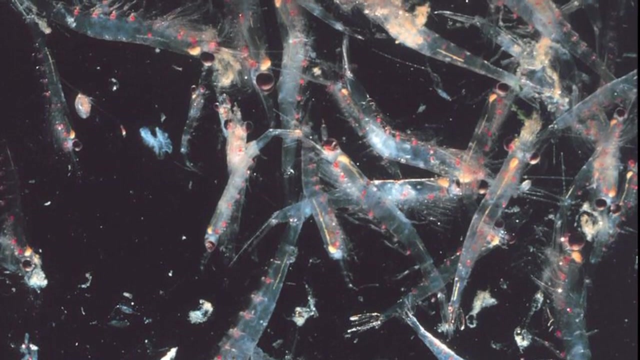 The name krill refers to about 85 species of free-swimming open-ocean crustaceans. Krill can be found throughout the world's oceans. Since these crustaceans average only 2 inches in length, they are often found in large swarms. 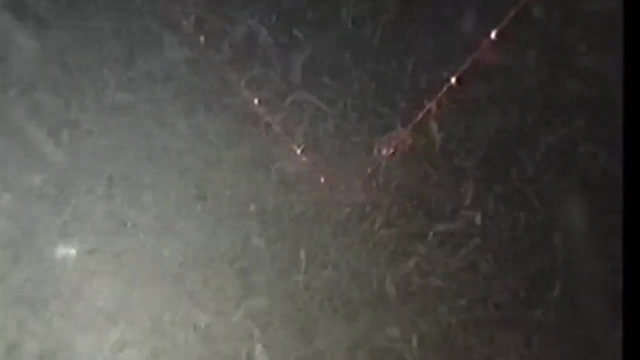 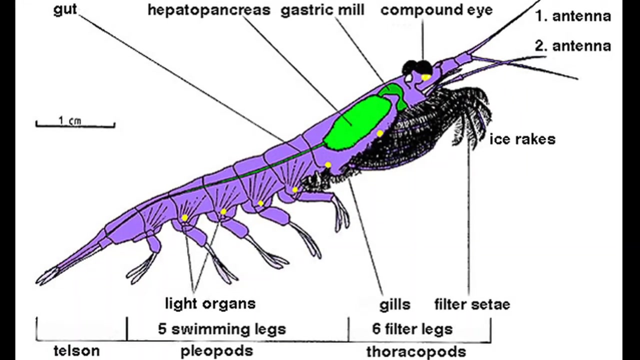 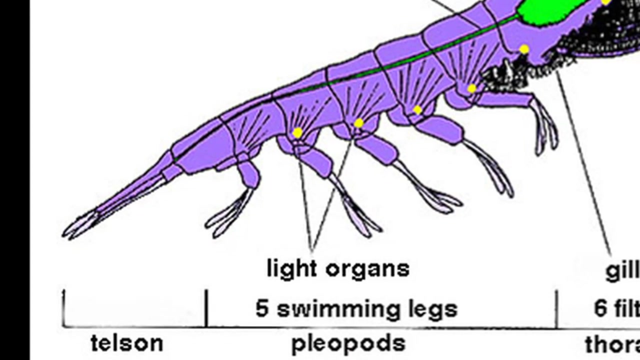 They must continually swim in order to maintain their position in the water column. They have a filamentous gill structure that increases their surface area for gas exchange. In almost all species, their body contains luminous organs called photophores that produce blue light. 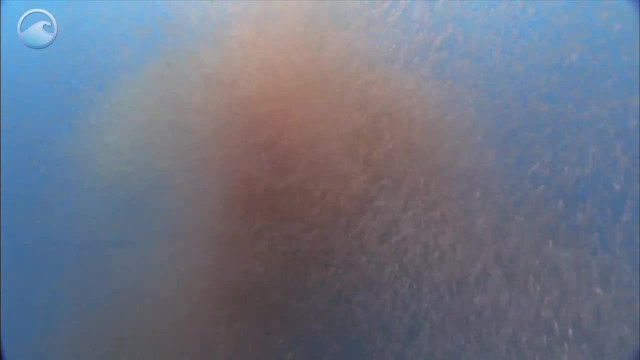 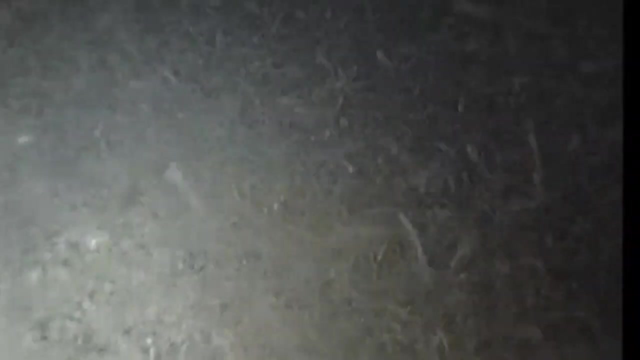 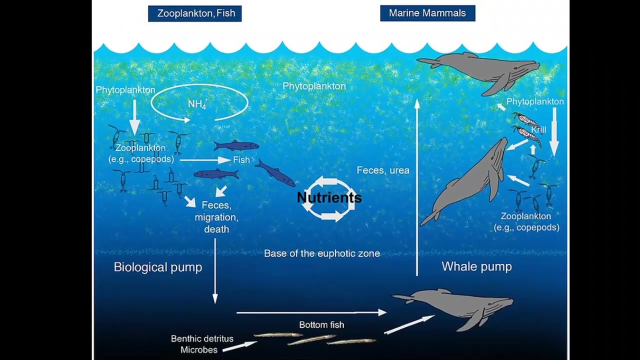 Krill go through a vertical migration every day. They move towards the ocean surface at night and back into deeper waters during the day. It is thought that they do this to avoid predation and increase feeding efficiency. Their migrations result in the extra benefit of transporting ocean nutrients. 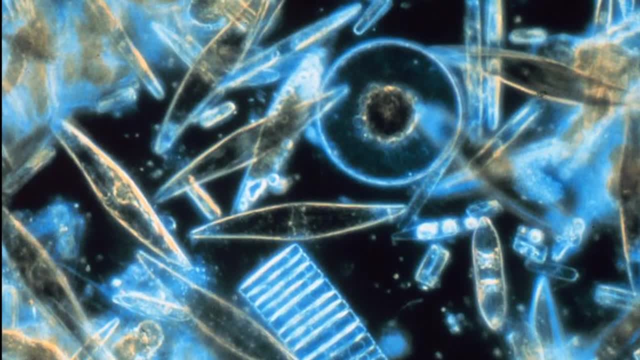 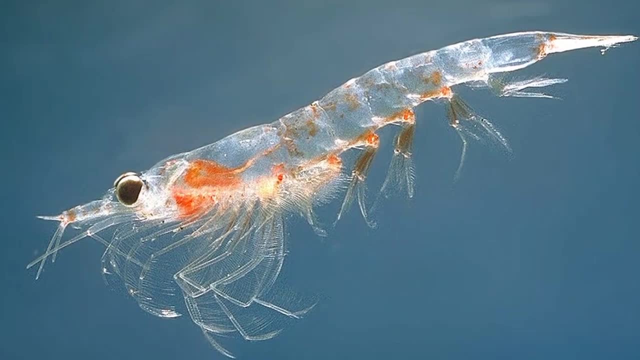 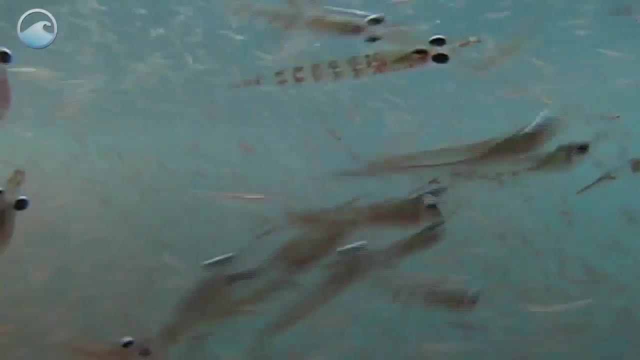 Most krill are filter feeders that primarily feed on phytoplankton. Their bodies are mostly transparent, so their digestive system is usually visible. Krill are consumed in countries like Japan and Russia. In the United States, krill can be found as supplements for things like joint pain. 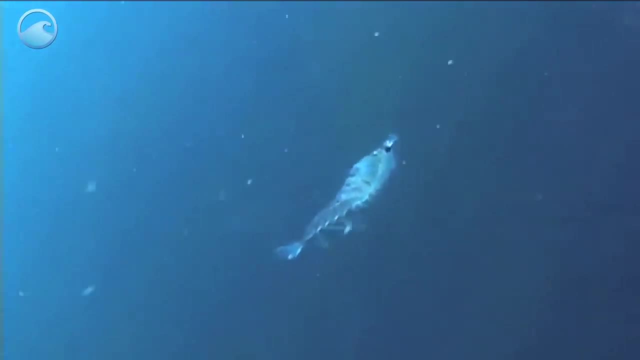 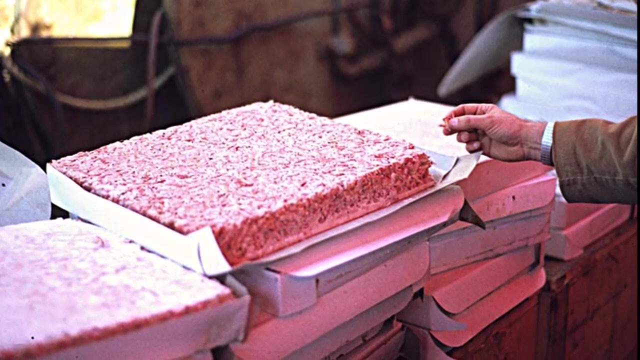 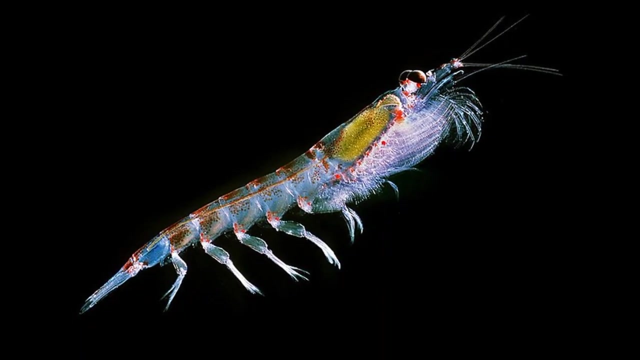 A lot of animals like whales, seals, squid and birds depend on krill to survive. Krill populations are threatened by commercial fishing and climate change. In the Southern Ocean, Antarctic krill are a keystone species. These krill have faced population declines due to ice loss. 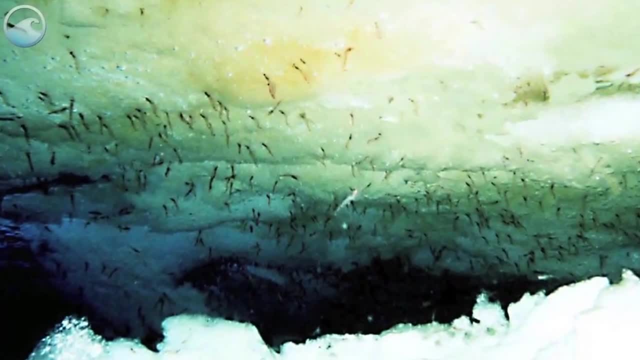 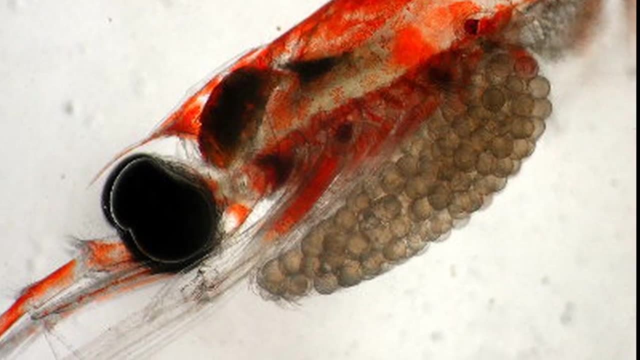 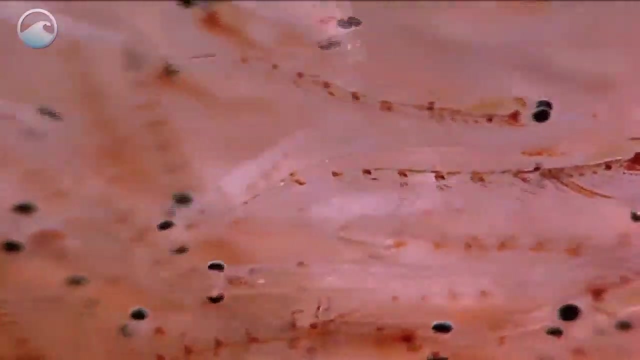 This is because the presence of ice provides habitat for their primary food source, ice algae. Methods of reproduction vary by krill species. For many species of krill, spawning occurs in deep waters. Females lay up to 10,000 eggs at a time. 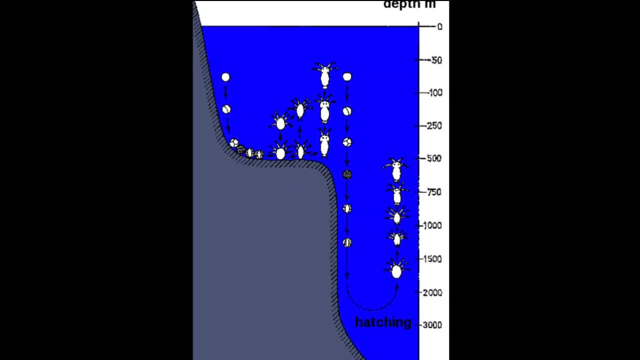 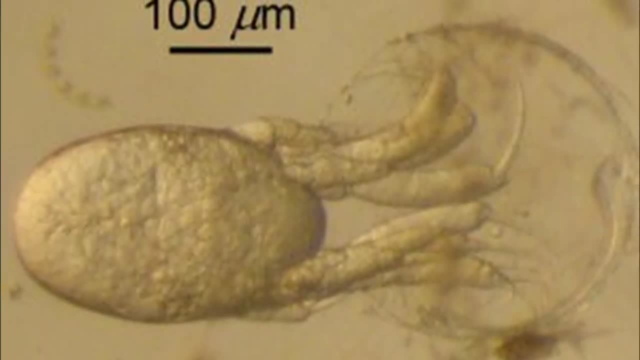 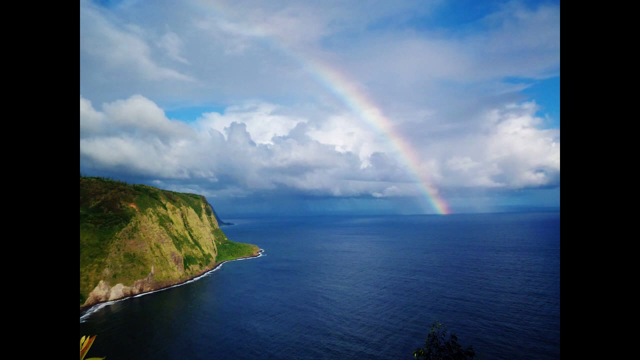 Their eggs sink and the resulting larvae eventually ascend to the surface to feed. Krill continue to molt and grow throughout their whole life cycle. Some krill species can live five or more years. For more marine facts, click the subscribe button.